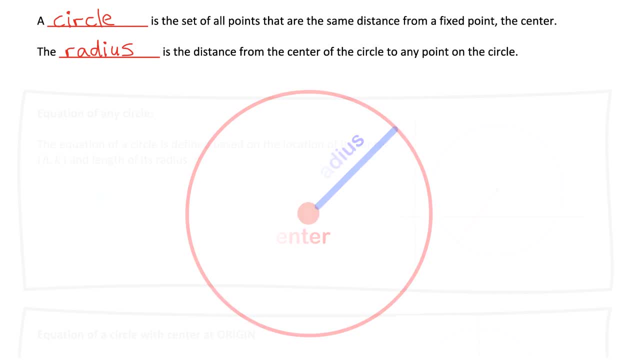 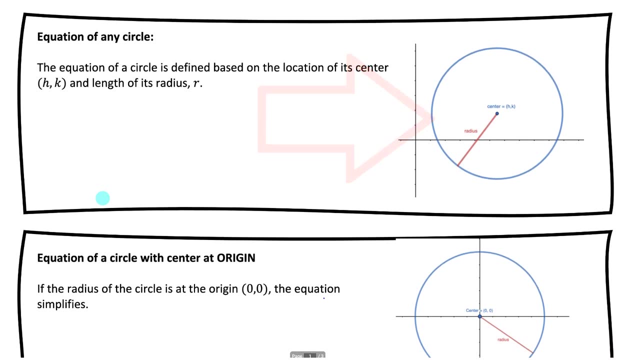 center of the circle, that fixed point to any other point on the circle. What I'm going to do next is show you the equation of a circle that is not centered at the origin and the equation of a circle that is centered at the origin, And then, after I show you the equations, I'll give you a. 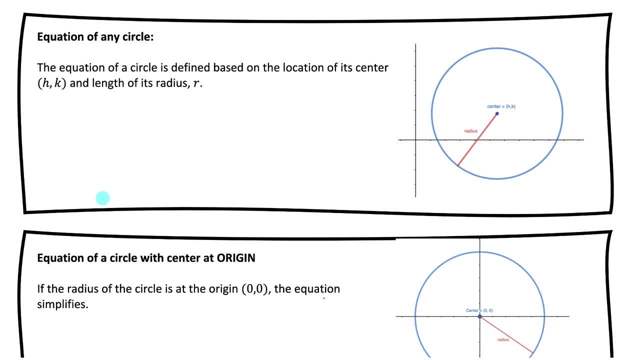 detailed explanation as to why the equation is able to describe the relationship between any xy point and the radius of the circle. So first of all, let's start with any circle. So the circle that could be centered anywhere doesn't have to be at the origin. In that case, we call the center 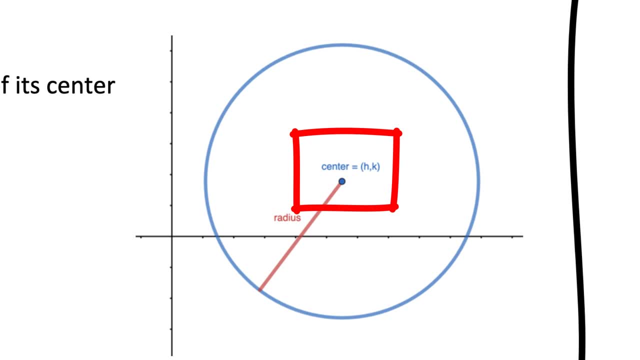 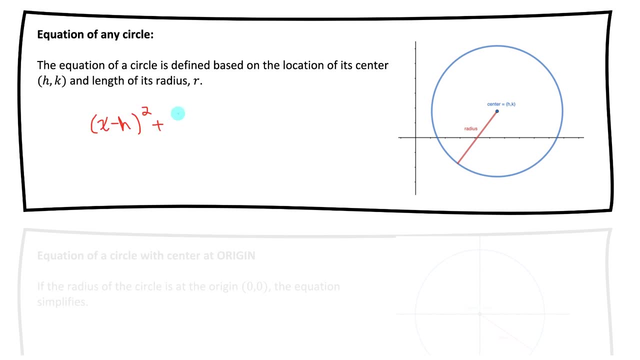 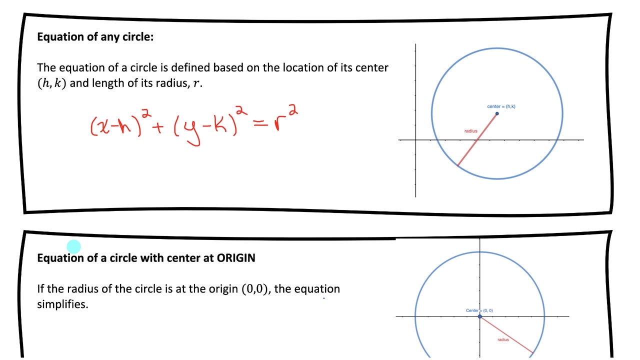 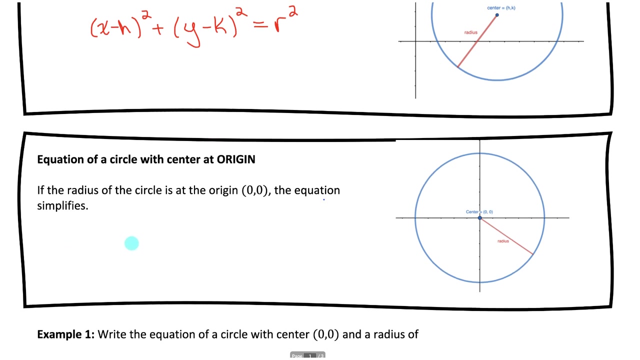 of the circle, point hk And the relationship between any xy point and the radius is: x minus h squared plus y minus k squared is equal to the radius squared If the circle is centered at the origin. that would make the h and k values zero, which means the equation would simplify to just: x squared plus y squared equals r. 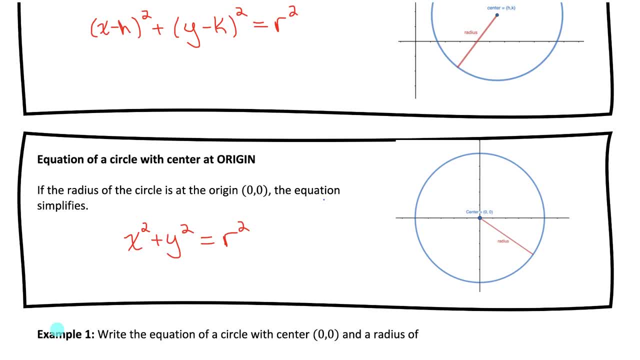 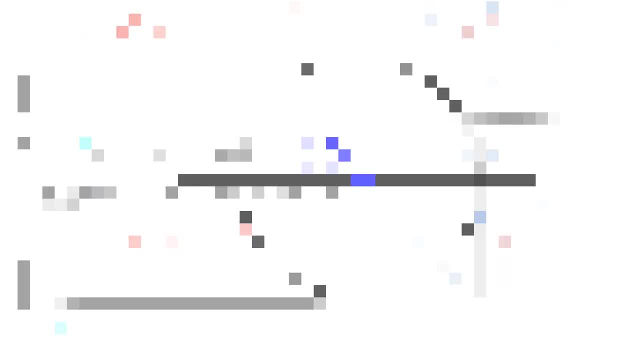 squared. Now, why do these equations describe the relationship between any xy point, the radius? well, maybe let's look at a more clear diagram of a circle. here I have a circle drawn that centered at the origin, So I have the center labeled as the point 00.. 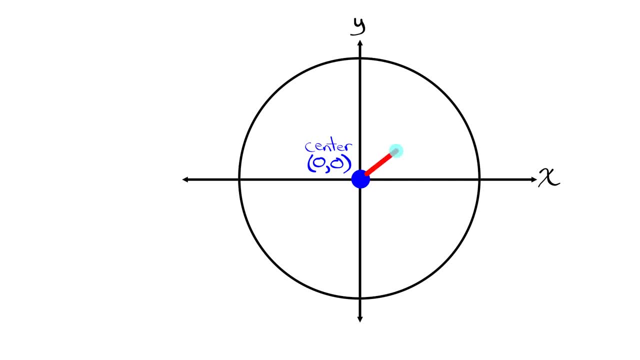 If you can imagine me drawing a radius from this center 00, to any point on the circle, so anywhere on the circumference of the circle, it would connect to the circle at some point xy. So I'll label this circle as point xy And I've drawn the radius. let me label that as r to represent the radius. 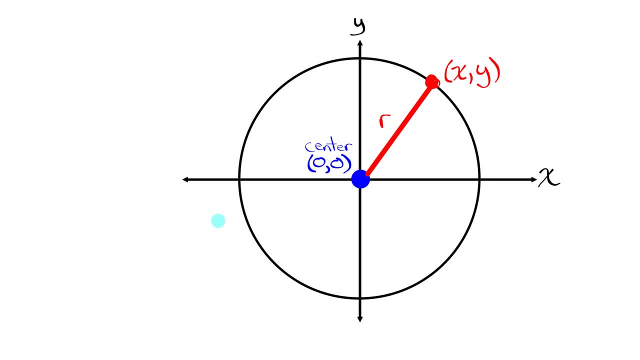 of the circle. Now, if I were to describe the relationship between this xy point and the radius, if I were to go from the origin to that xy point, I could travel x units parallel to the x-axis and then y units parallel to the y-axis. So let me label those side lengths as x and y. 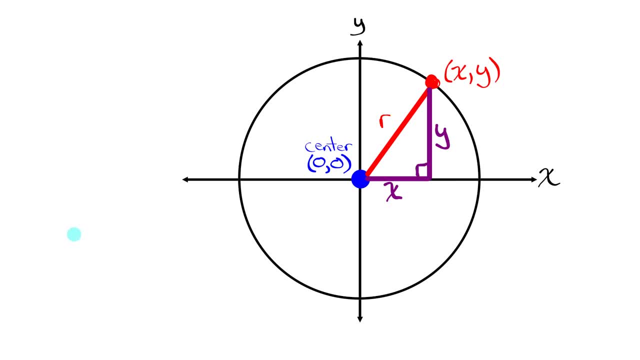 and notice what I've created here is a right angle triangle. And what do we know about the relationship between the sides in a right angle triangle? We know that the sum of the squares of the shorter two sides, so x squared plus y squared, is equal to the square of the longest side. 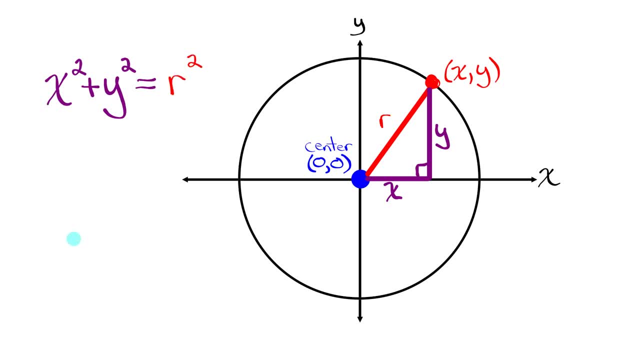 In this case the longest side is the radius, so it's equal to the radius squared, And this is the equation of a circle: x squared plus y squared equals r squared, And that relationship between the xy point and the radius is called the radius squared, And this is the equation of a. 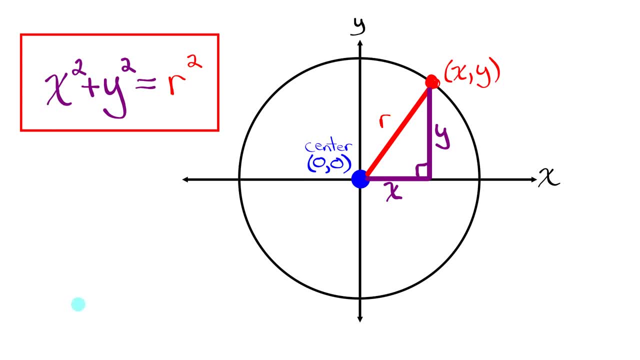 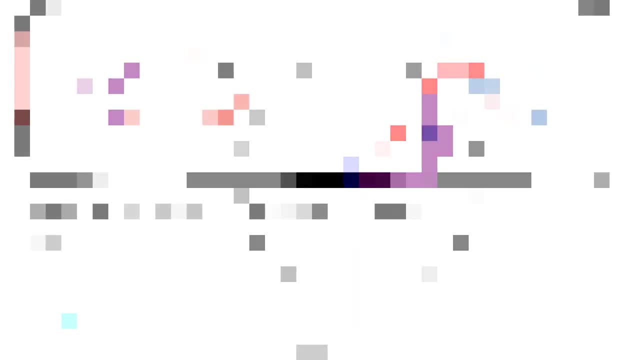 And the radius holds true for any x, y point on the circumference of the circle if the circle is centered at the origin. So hopefully now you can understand where this equation of a circle comes from. Let's now practice writing the equation of a circle. 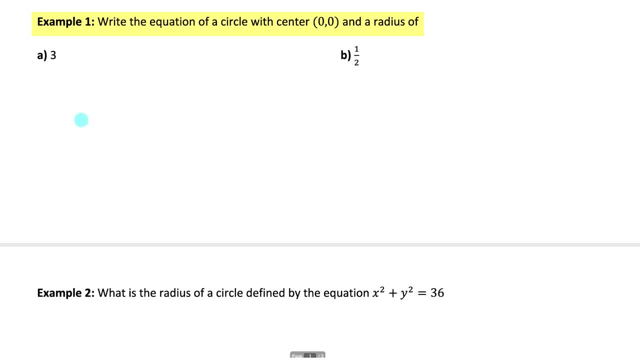 Example 1 says: write the equation of a circle with center 0, 0 and a radius of, in part a, 3.. So it gives us the radius, And when we write the equation of a circle, remember we write it in the format of x squared plus y squared. 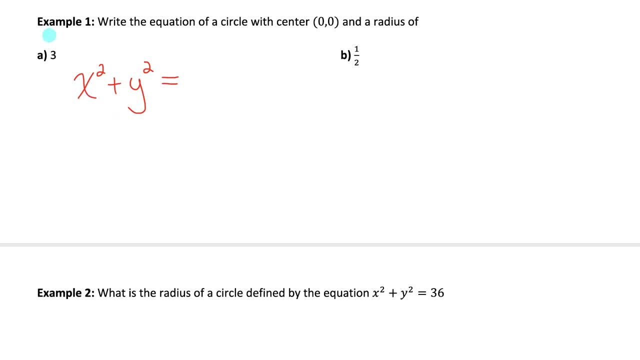 equals the radius squared, And in this case we know the radius is 3.. So we would write it as 3 squared, And whenever we're expressing our final answer for the equation of a circle, we'll need to simplify the radius squared. 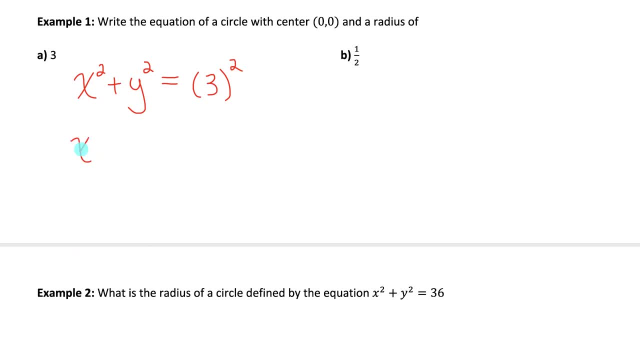 So we'll need to actually evaluate what 3 squared is. So in this case, the equation of the circle would be: x squared plus y squared equals 9.. And that would be our final answer for the equation of that circle. Let's try another one. 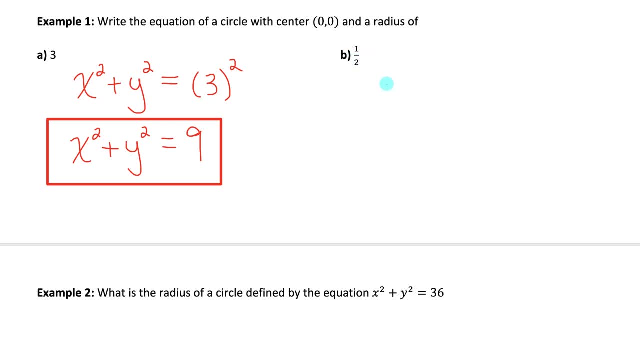 This time the radius of our circle is a half, So when I write the equation of this circle, it would be: x squared plus y squared equals a half squared. And remember, when the base of your power is a fraction, what we need to do is apply the exponent to the numerator and the denominator. 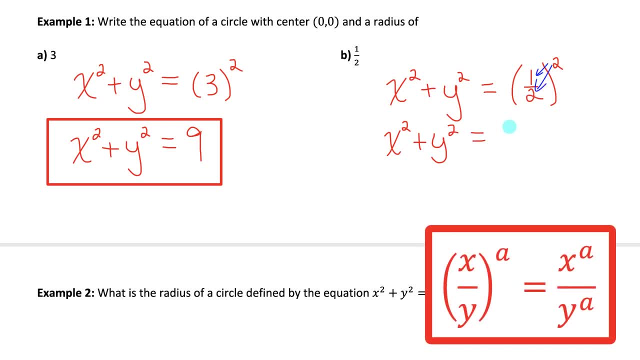 So I need to square the 1 and square the 2.. So 1 squared is 1 and 2 squared is 4.. So the equation of this circle is: x squared plus y squared equals a quarter. Let's move on to example 2,. 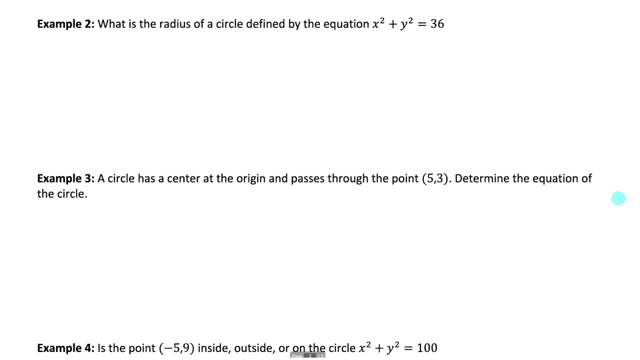 where. this time it gives us the equation of the circle and it asks us for what the radius is. Example 2 says: what is the radius of a circle defined by the equation x squared plus y squared equals 36?? First thing you need to remember is the number that you see on the right side of the equation. 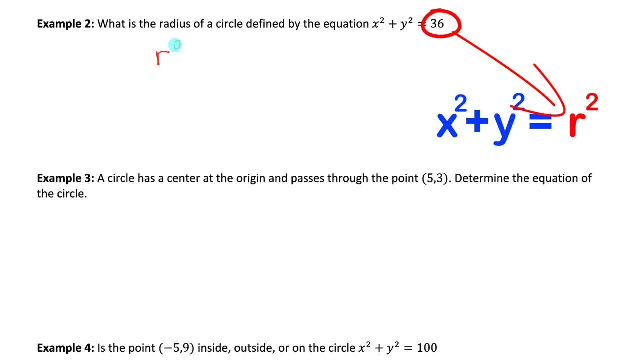 is what the radius squared is equal to. So in this case the radius squared is 36.. If we're interested in the radius, we'll have to isolate r. On the left, r is being squared, So to isolate r we have to do the inverse of squaring. 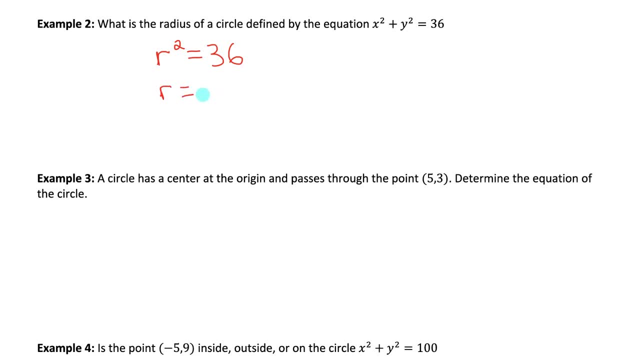 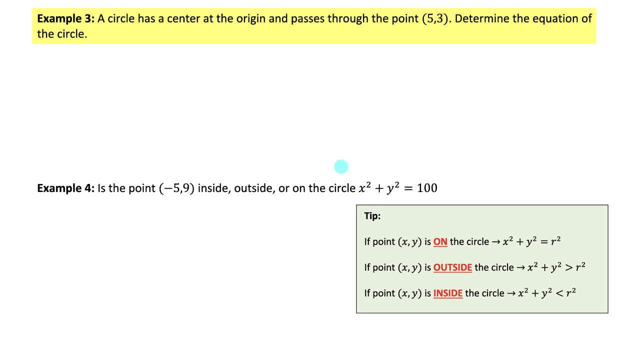 which is square rooting. So r would be equal to the square root of 36,, which is 6.. So the radius of this circle is 6 units. Example 3 says a circle has a center at the origin and passes through the point 5,. 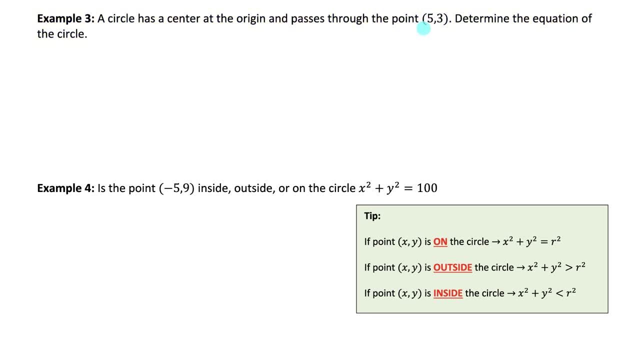 3. Determine the equation of the circle. So this time it gives us an xy point, that is, on the circumference of the circle. So, in order to determine the equation of this circle, let me start by writing out the general formula for the equation of any circle centered at the origin. 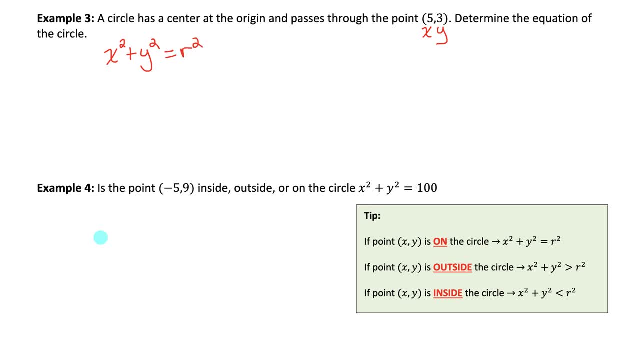 x squared plus y squared equals r squared. In order to write the equation of this specific circle, I'm going to have to solve for what r squared is equal to. To do that, I will sub my xy point in for x and y. 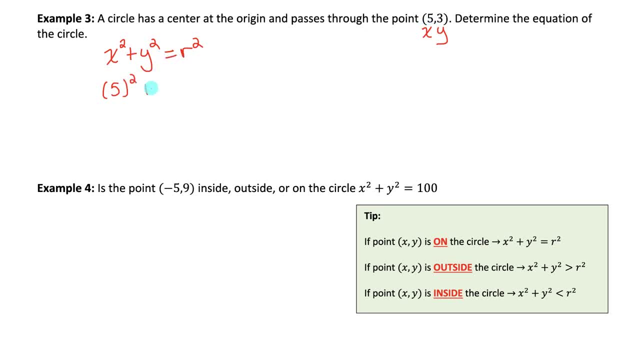 That will give me 5 squared plus 3 squared is equal to r squared. 5 squared is 26.. 3 squared is 9.. So I can see that r squared is equal to 34.. Now I'm not actually interested in what r is equal to. 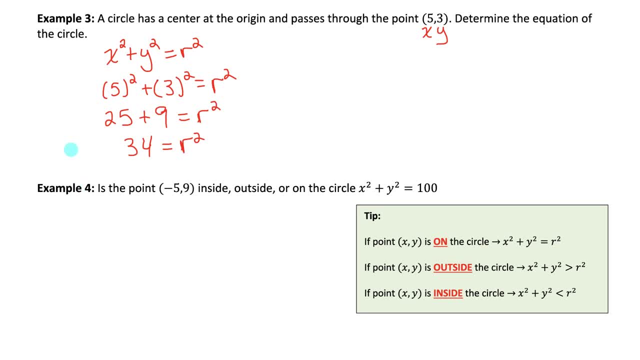 I don't care what the radius is. The question doesn't ask for it, It just wants the equation of the circle. And in the equation of the circle, I just need to know what the r squared value is, And I have it. 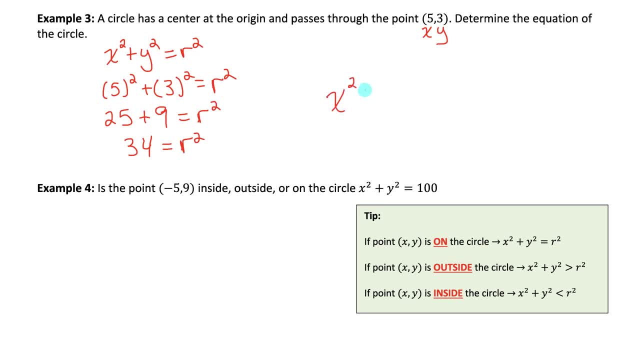 It's 34.. So I can write my final answer: x squared plus y squared equals r squared. So I can write my final answer: x squared plus y squared equals r squared, which is 34.. So this is the equation of the circle centered at the origin, with 0.53 on its circumference. 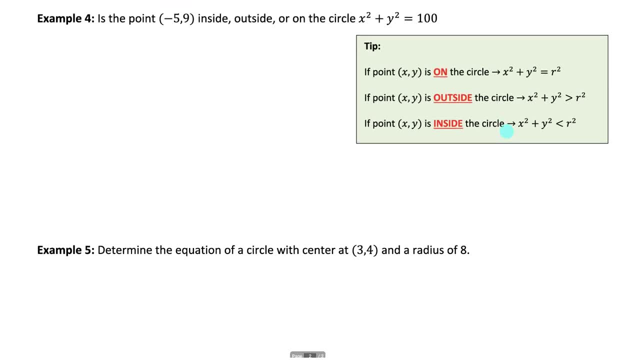 The next question is a very typical question for this section of the unit. It wants to know if a point lies inside, outside or on a specific circle. Let's look at the general rule for determining if any given point falls inside, outside or on any given circle. 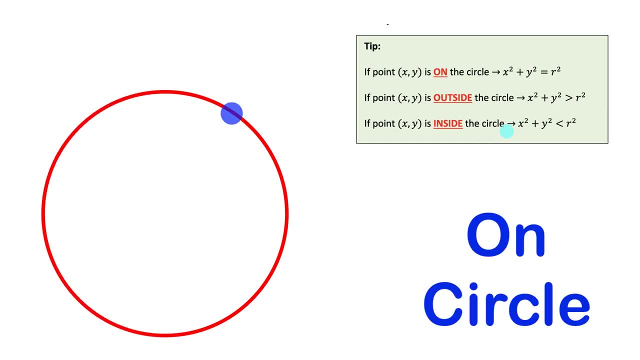 If the given xy point is on, then x squared plus y squared would be equal to the radius squared that's given in the equation of the circle. If the xy point is outside the circle, then x squared plus y squared would be greater than the given r squared value. 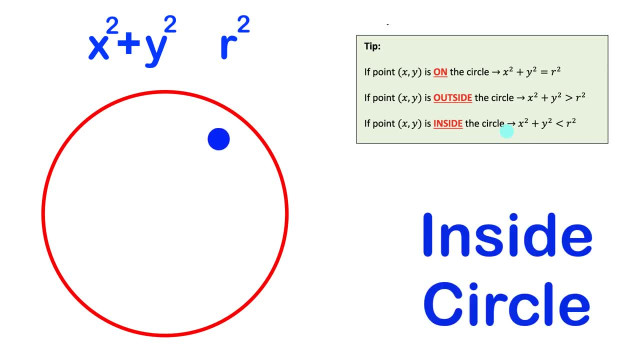 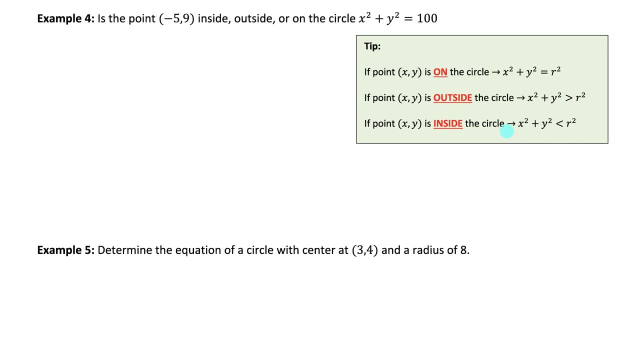 And if point xy is inside the circle, then x squared plus y squared would be less than the r squared value that's given by the circle. Let's try it out for the information we need. It says: is the point inside, outside or on the circle? x squared plus y squared equals 100?? 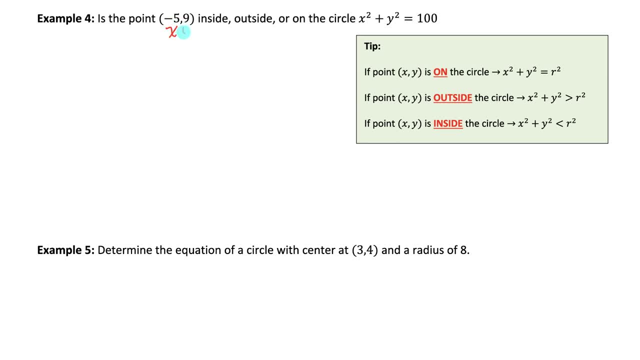 What we have to do is sub in the point for x and y into the equation of the circle that we have and see if x squared plus y squared is less than, equal to or greater than the 100 value that is, the r squared of this circle. 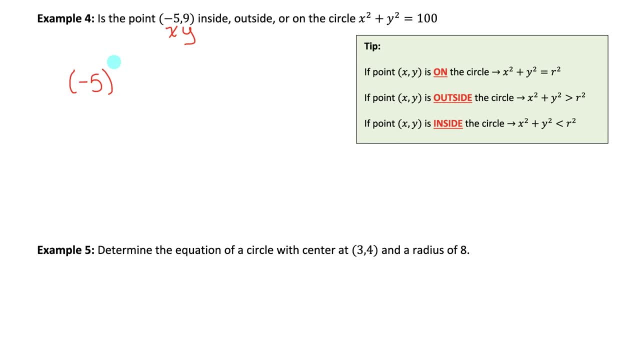 So we're checking What is the relationship between negative 5 squared and 9 squared in comparison to this 100 value, that is, the r squared value of this circle. Is it greater than, less than or equal to? So I just put an equal sign with a question mark above. 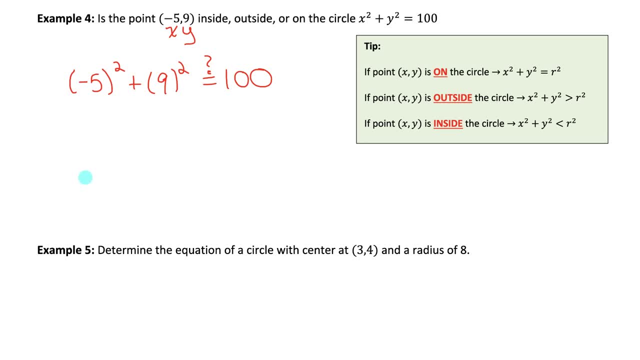 and we're going to test out to see the relationship between the left and right side of this equation. On the left, I have 25 plus 81.. And how does that relate to 100? Well, 25 plus 81 is 106. 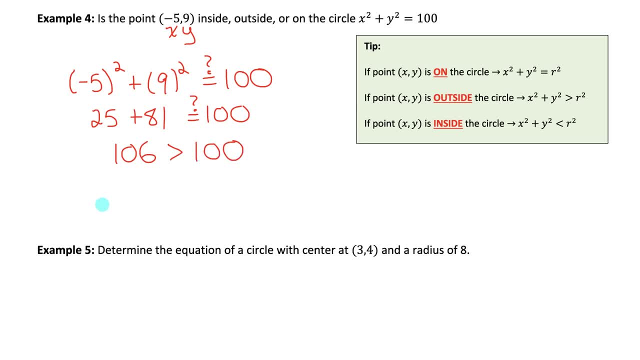 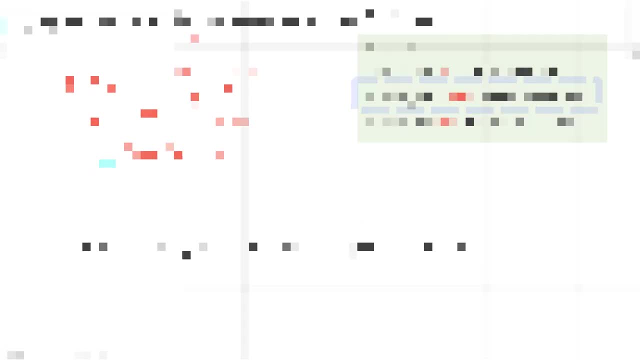 I know that is greater than 100.. That tells me that the point negative, 5, 9, is actually outside of the circle. that's given. Let's verify that in Desmos. So if I graph the equation of the circle, x squared plus y squared equals 100,. 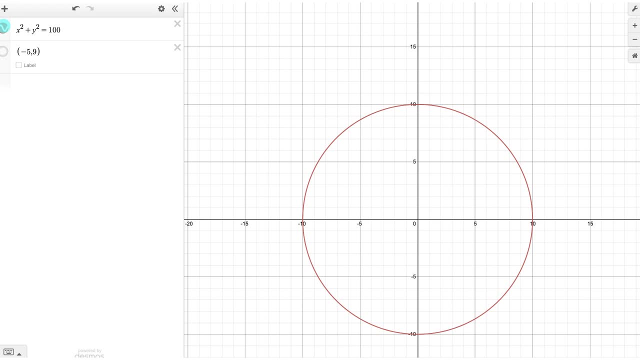 we have it right here. And if I were to plot the point negative 5, 9,, we figured out that its x squared plus y squared value would be bigger than 100.. It was 106, so that should tell us that it's outside the circle. 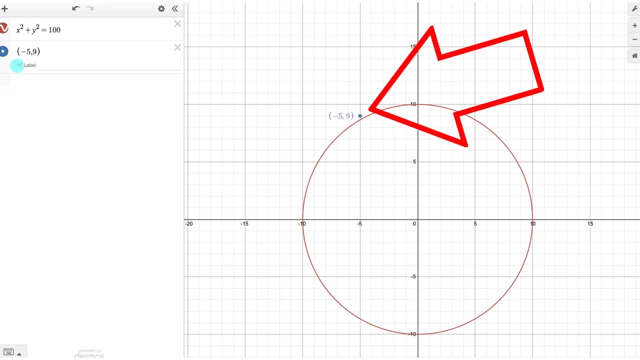 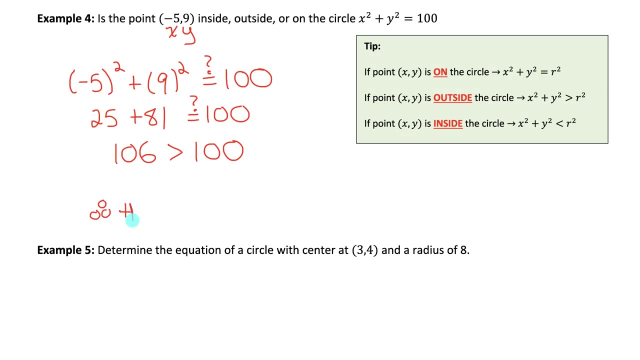 And if I plot it, notice that that point negative 5, 9 is just outside the circle. So we got the correct answer. We should summarize our answer by saying: therefore, the point negative 5, 9 is outside of the circle. 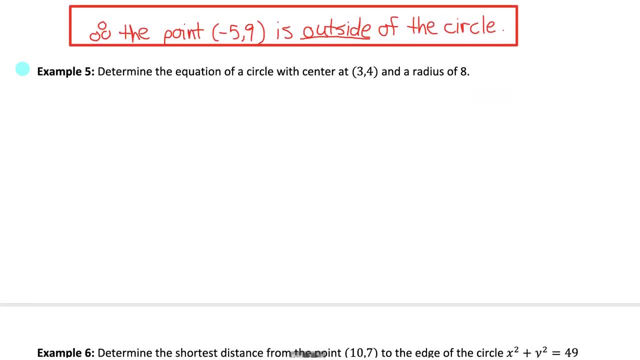 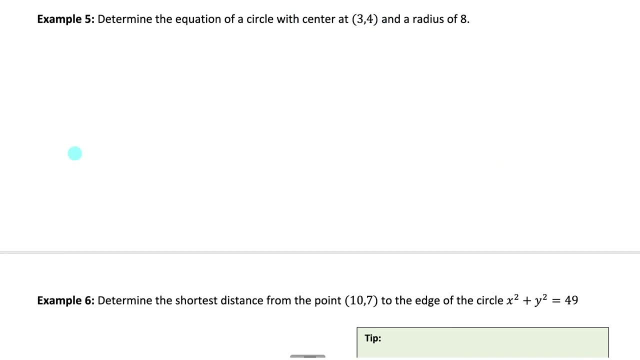 Let's move on to question number 5.. This is the first time we're finding the equation of a circle where the center is not at the origin. So let me remind you what the equation of a circle not centered at the origin looks like. 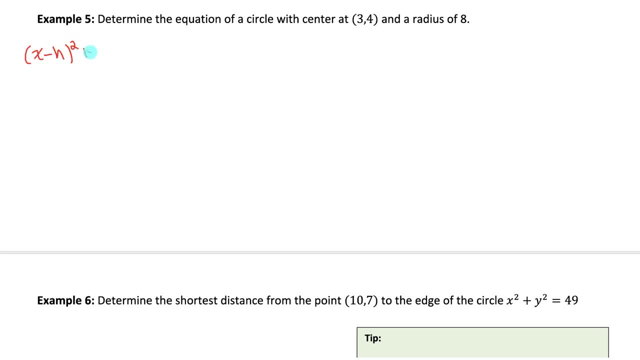 It is x minus h squared, plus y minus k squared, equals r squared h and k. that you see in this equation is the center of the circle. So in this case, 3, 4 are our h and our k values, And it tells us the radius r is 8.. 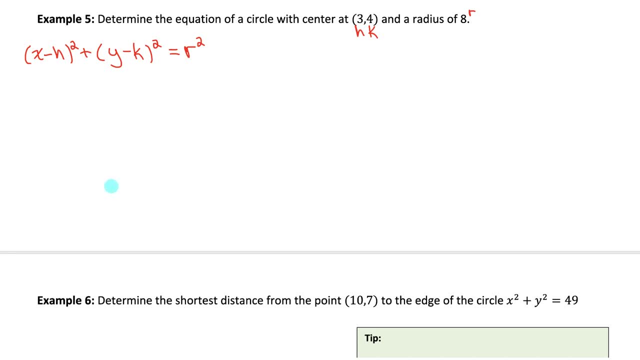 So to write the equation of the circle, I'll just plug in my h, k and r and then I'll have the equation. The answer would be x minus 3 squared plus y minus 4 squared equals 8 squared. And remember when writing the final answer for the equation of a circle: 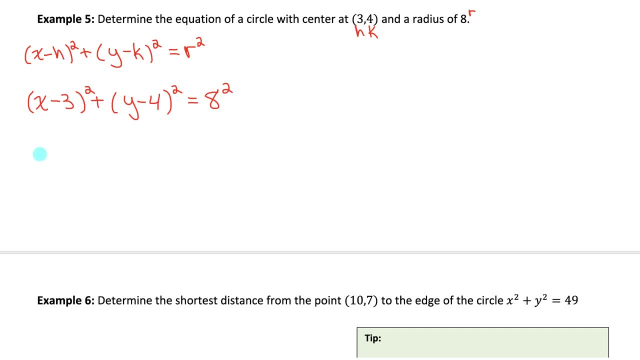 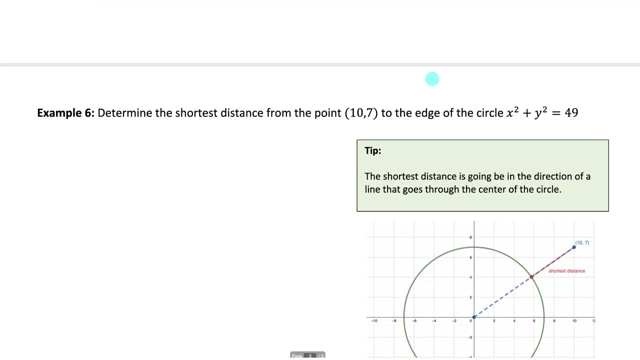 we need to simplify the radius squared, So I'll actually have to evaluate 8 squared. My final answer will be: x minus 3 squared plus y minus 4 squared equals 64.. And now let's go on to the last question of the lesson. 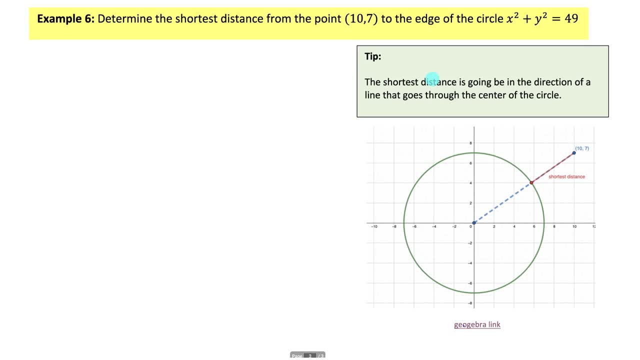 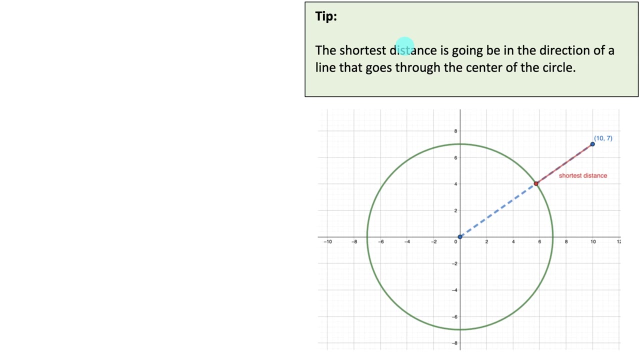 It says to determine the shortest distance from the point 10, 7 to the edge of the circle. x squared plus y squared equals 49.. Now you can see in this diagram I have the point 10, 7 labeled and I have the graph of the circle. x squared plus y squared equals 49.. 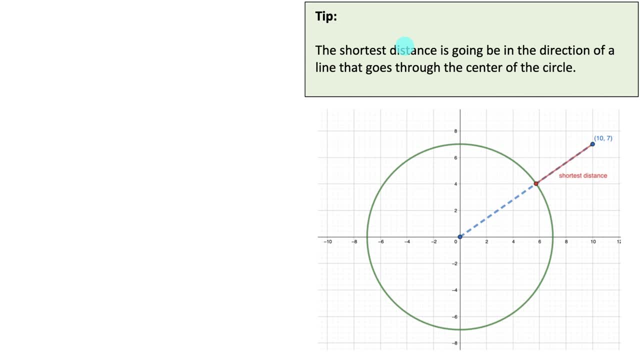 Now I've given you this so you can visualize what we need to do, and then we'll algebraically calculate it. And I put an important tip here. It says that the shortest distance from a point to a circle is always going to be along a line. 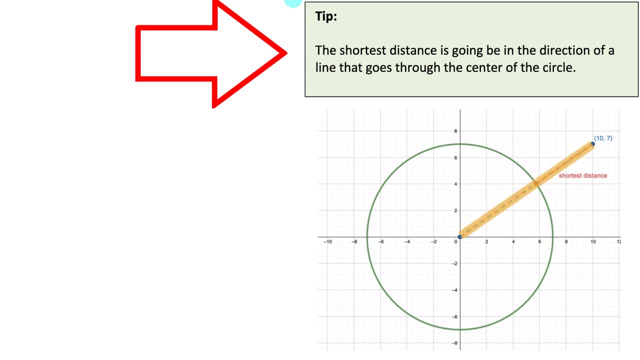 that goes from the point along a line that goes through the center of the circle. So the first thing we're going to do is calculate the distance from that point 10, 7- to the center of the circle, And we can do that using your distance formula. 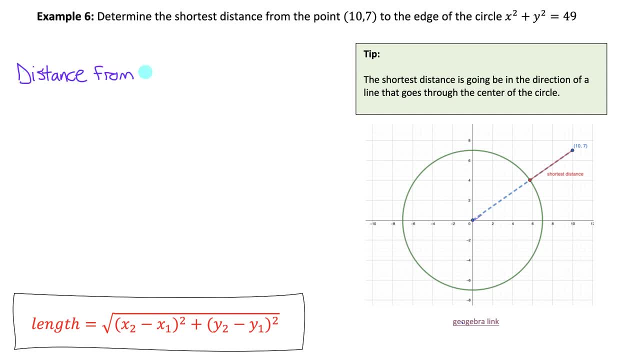 So I'll start by finding the distance from the point 0, 0, which is at the center of the circle, to the point 10, 7.. And using the distance formula, I know it will be equal to the square root of the difference in the x quarter.